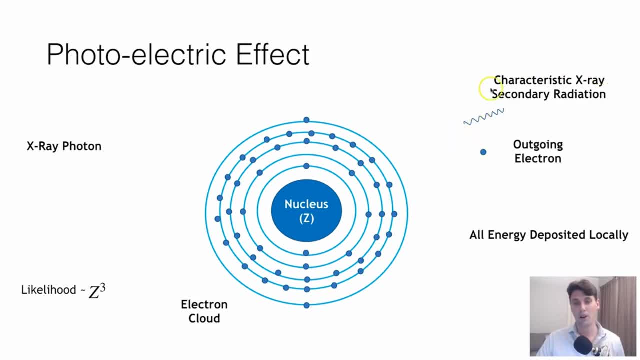 secondary X-ray is emitted. But what's important to remember is that right here we have an X-ray and an electron, But those are both going to deposit their energy fairly locally. So we can think about it to first order: As the X-ray comes in, it interacts with the matter And then it deposits its 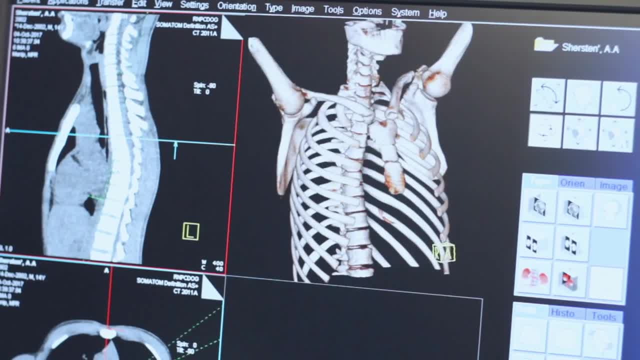 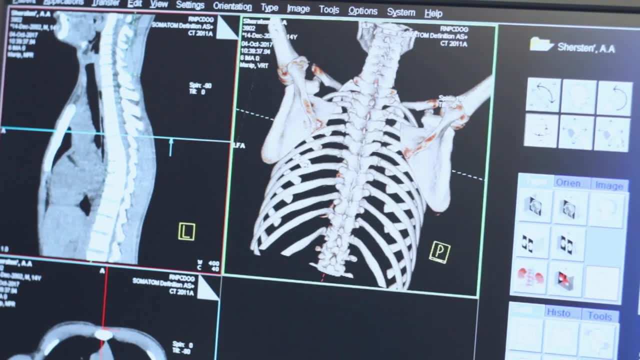 energy locally. So this is nice from the perspective of if we want to generate contrast in an image, it's nice that we can have some energy deposited locally And then we can basically make a map of that, And we'll talk about that in additional lectures. 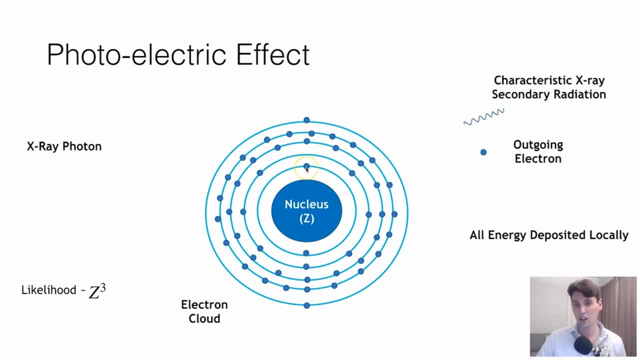 But one thing to keep in mind here is that this was an inner shell electron that was having this interaction And that's very much driven by what's in the nucleus, namely what's the atomic number, how many protons are in the nucleus. So the likelihood of this interaction, 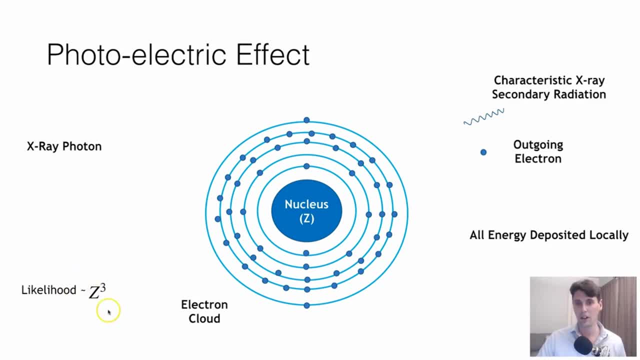 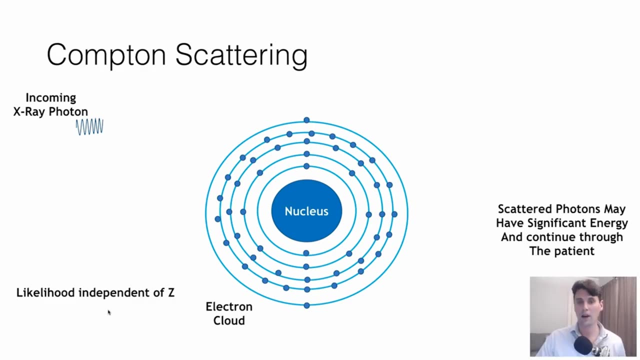 goes like Z cubed, or how many protons are in the nucleus cubed. So things that have more protons are going to have higher contribution of photoelectric effect when they're interacting. So we'll keep that in mind. And then the other thing is Compton scattering. So Compton scattering is the second dominant. 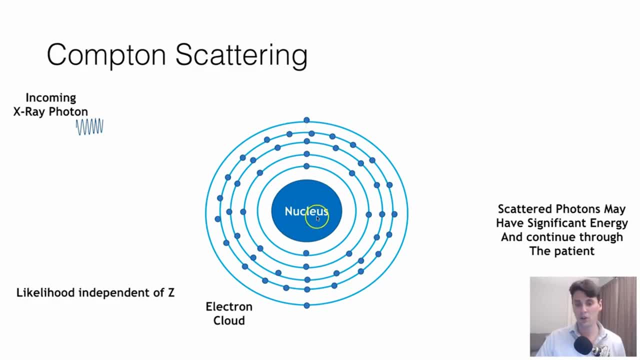 effect in X-ray imaging. So in this case, again we have the nucleus and then we have an electron cloud. In this case it's the photon coming in and the photon is interacting with an outer shell electron And because it's so far from the nucleus, the likelihood 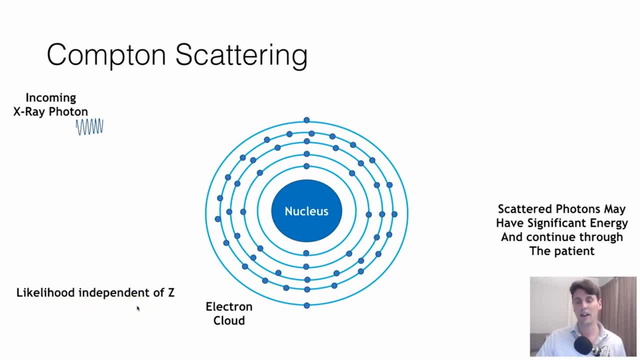 of the interaction is zero. It's independent of Z, So it's not really dependent on what's in the nucleus. Photon comes in, It knocks the electron out And then the photon goes out in the opposite direction in order to conserve momentum. 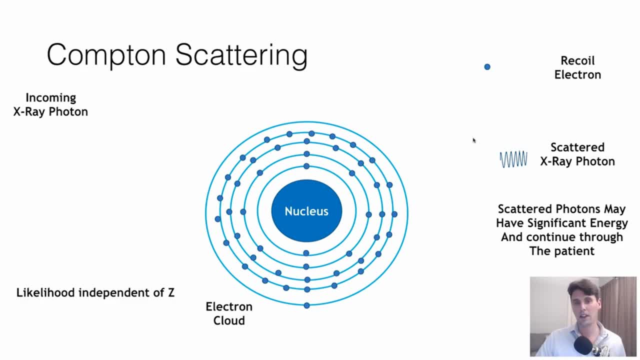 So what's important to remember here is that, unlike in the photoelectric effect, the energy is not all deposited locally. So this scattered photon may still have a significant fraction of the energy of the incoming photon, And that can still travel through the patient and potentially could have a second 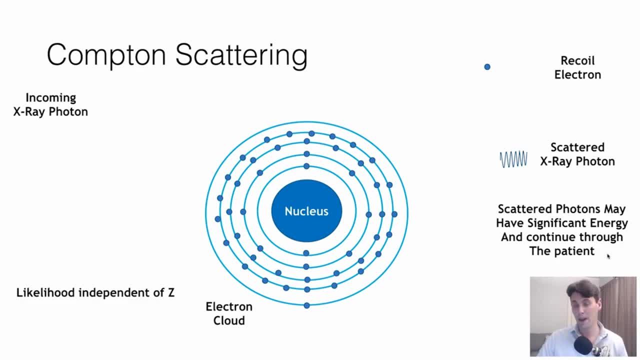 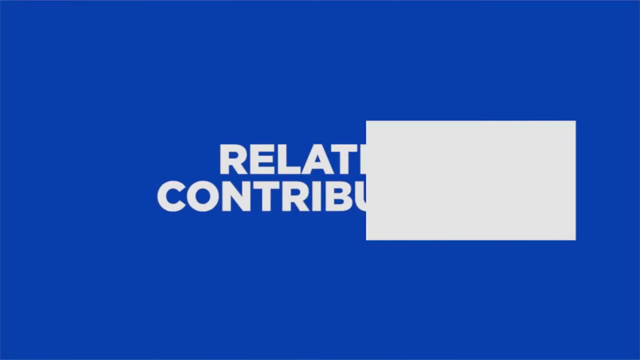 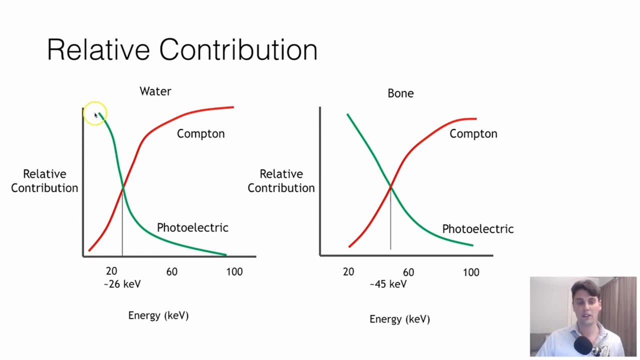 Secondary scatter effect or potentially could get measured on the detector. So we've covered the two major interactions, photoelectric and Compton, And if we look at the relative contribution of those two we can see a plot like this where this is the relative contribution. So these right here are saying at low energies it's all the interactions. 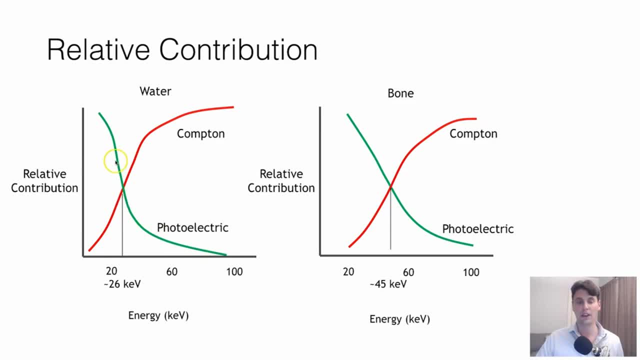 are really dominated by photoelectric. Photoelectric is in green here and Compton is in red. And then at high energies, everything is dominated by photoelectric. And then at high energies, everything is dominated by photoelectric. And then at high energies, everything is dominated. 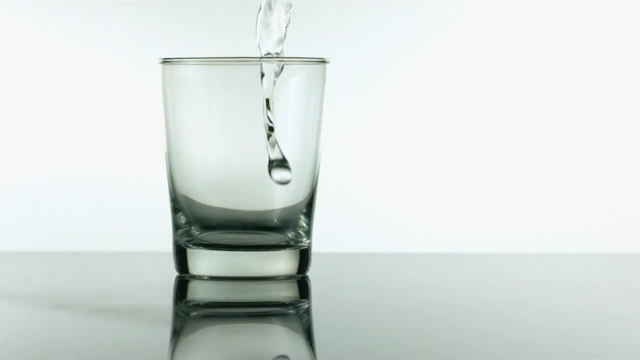 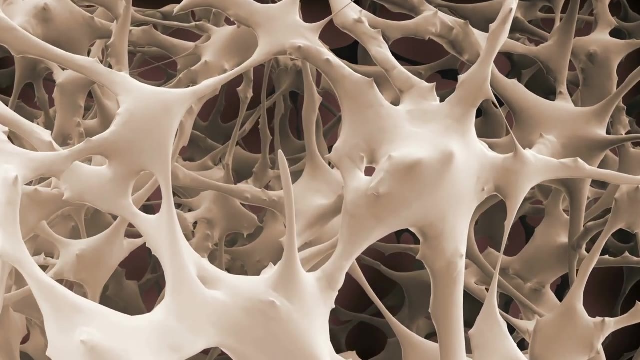 by Compton, And that's true for these different types of material. The body can well be approximated as a bag of water for the soft tissue sake, And then the bone in the body here shows a similar behavior, but the point at which they cross over is a little bit higher. So photoelectric. 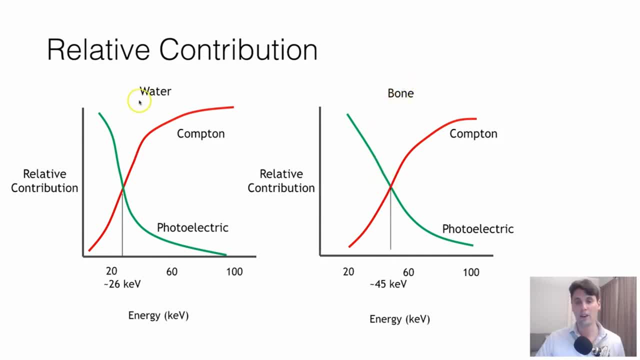 is dominant for more of the time in bone than in water. So up to 26 keV photoelectric is dominant in water And it's up to 45 keV that photoelectric is dominant in bone. So that's what we're talking about here. We just talked about the fact that the photoelectric effect 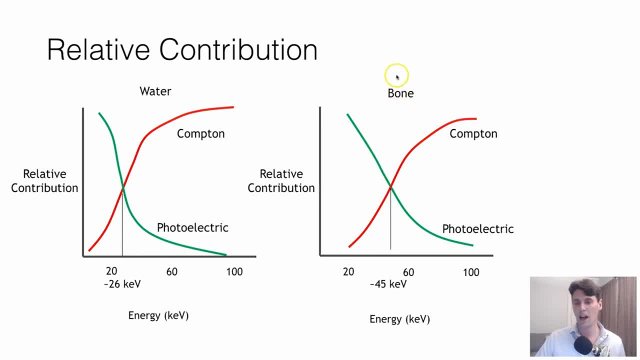 is strongly dependent on the Z and bone has a much higher Z. For instance, the calcium in the bone has a much higher Z, many more protons, than in water. So that's the fundamental relationship that we want to try and remember is at low energy, photoelectric is dominant. 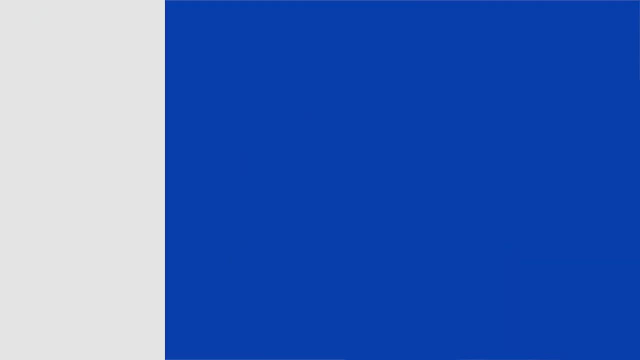 and at high energy, Compton is dominant. So just again to summarize really, take these points home: Photoelectric dominates interactions with water, And then at low energy, photoelectric is dominant, And then at high energy, Compton is dominant. So just again to summarize really. 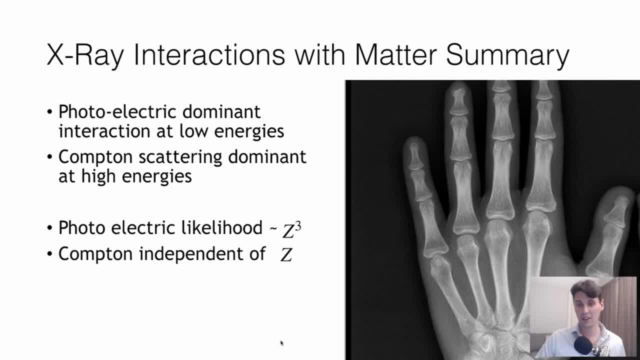 take these points home. Photoelectric dominates interactions at low energies, Compton will dominate interactions at high energies. And then the likelihood of these interactions: for photoelectric it's dependent on Z, cubed, And for Compton it's dependent on Z And. 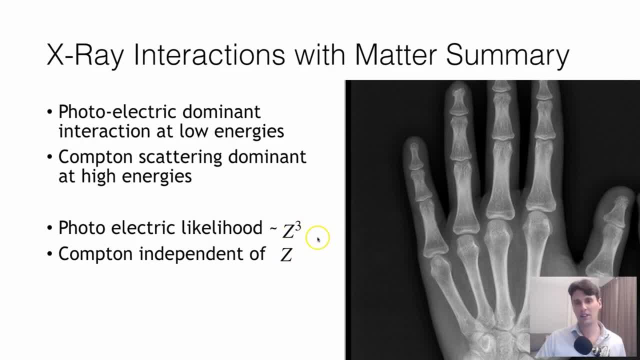 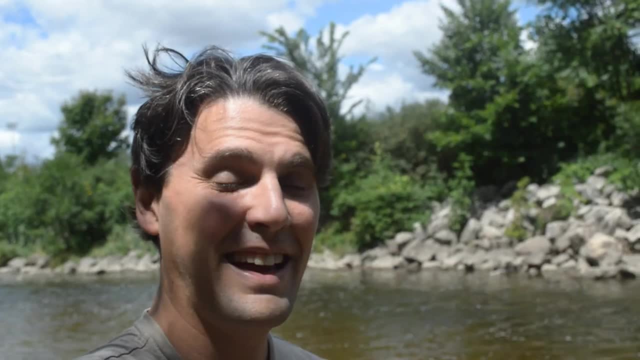 what does that tell us? It tells us that x-rays and x-ray imaging we're going to have really good contrast for things that are higher Z, like bone. So bone imaging on standard x-rays comes out really nice with really fine contrast. So thanks for sticking around, guys, and we'll see you in the next one. It's a summary on x-ray interactions with matter.